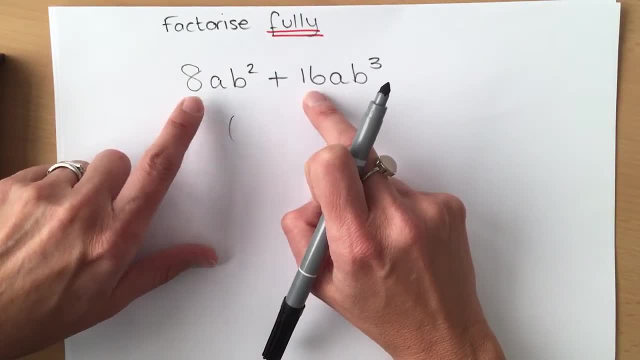 So we need to be looking at the numbers to start with. So we need to be looking at 8 and 16 and we need to be thinking about the highest common factors, So we need to take the biggest factor of 8 and 16.. 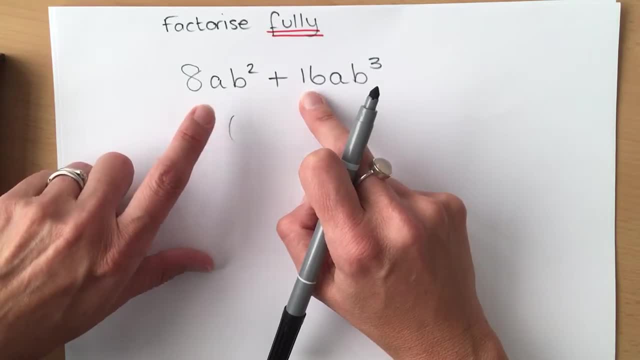 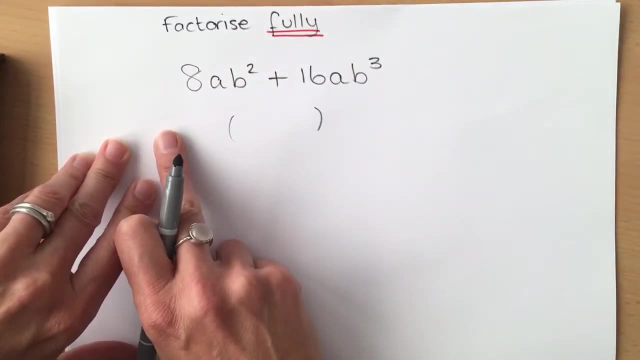 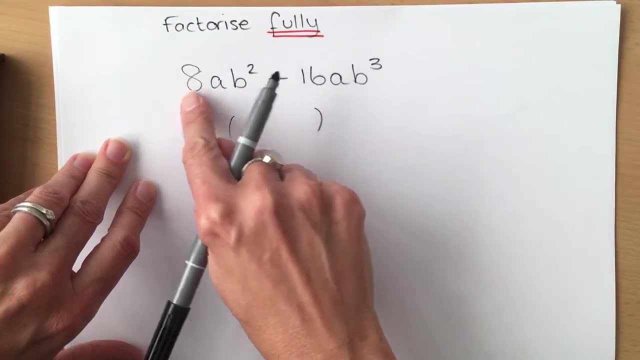 Now the factors of 8 and 16 are 2 and 4 and 8.. Now it says factorise fully. so if you put 2 outside the bracket you haven't factorised fully. If you put 4 outside, you haven't factorised fully. so you need to take the biggest factor of 8 and 16, which is 8.. 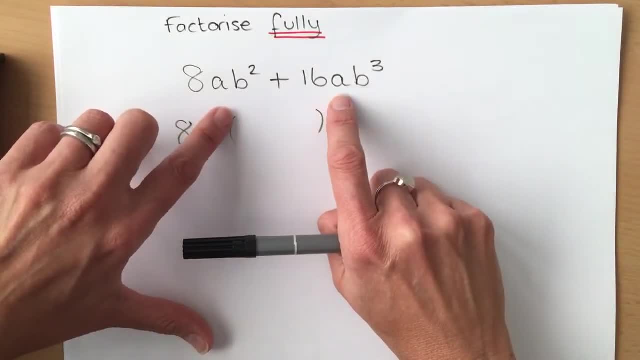 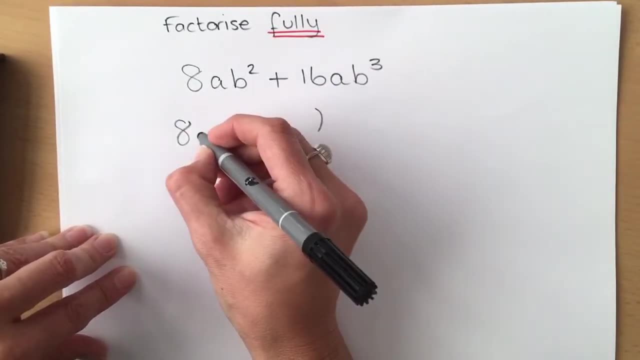 Then we need to move on to the A. OK, the biggest factor, The biggest factor of A I can take out, is A from here and A from there. So I'm going to take an A outside my bracket And then we move on to the other letter, B. 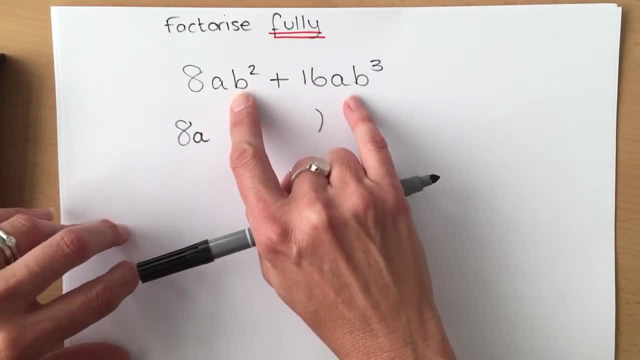 OK, we have a B squared and we have a B cubed. Now the highest power that I can take out from both- that's important, from both- is B squared. I can't take B cubed out which is in here, because there isn't a B cubed here. 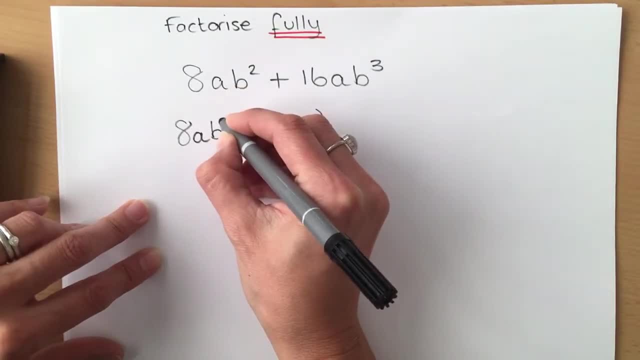 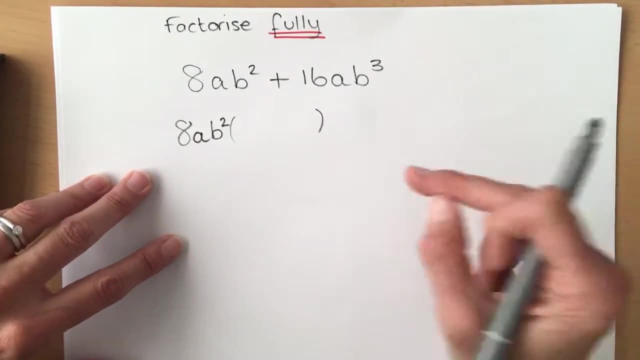 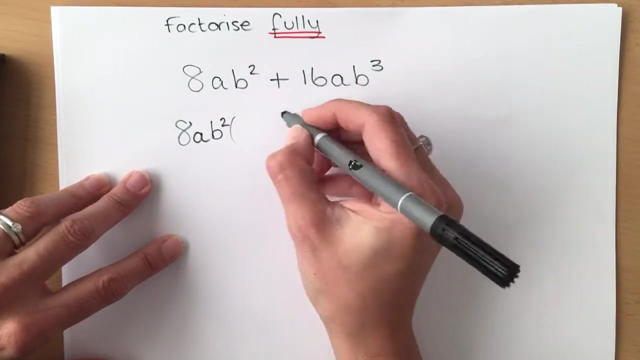 So the biggest power of B I can take is B. So there's B squared. OK, Now I have to work backwards and think: what am I going to put inside my bracket? Well, first of all, I'm going to take this plus sign and put it down here. 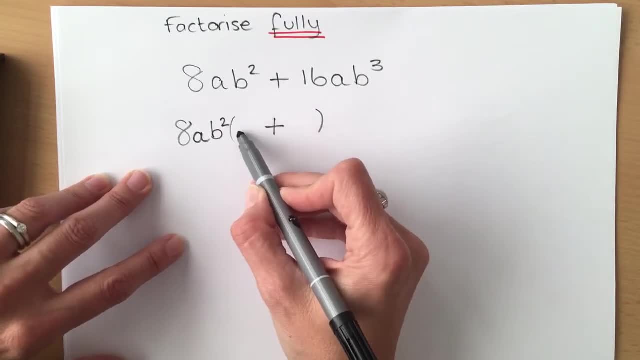 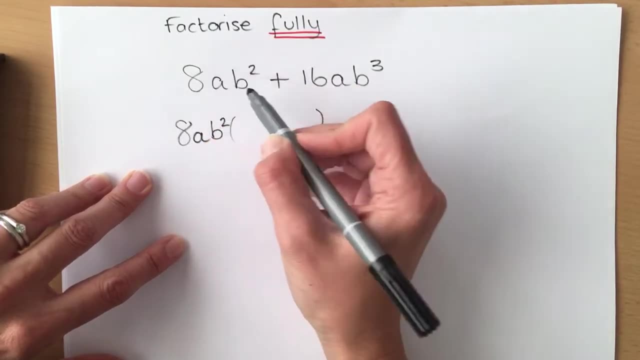 Then I've got to think about what I'm going to put here, Because I need to multiply this value here by 8ab squared and get 8ab squared. Well, if I need to multiply 8ab squared, Okay, Okay. 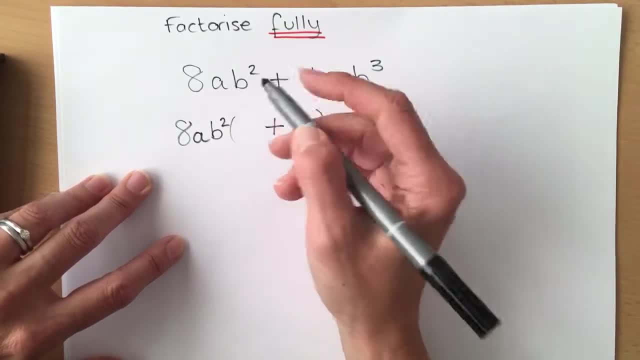 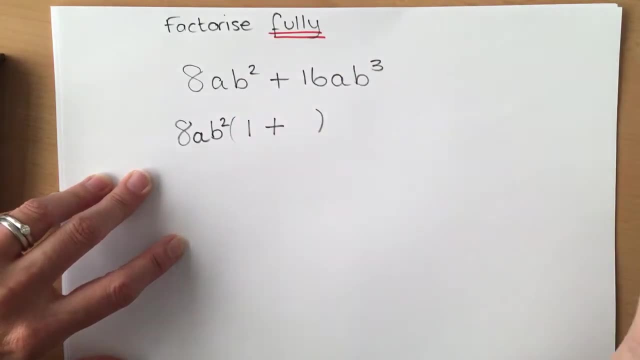 8ab squared by something and get the same answer: 8ab squared. The only thing I'm going to be multiplying it by is 1.. Because 1 times 8ab squared is 8ab squared. Now, moving on to this bit. 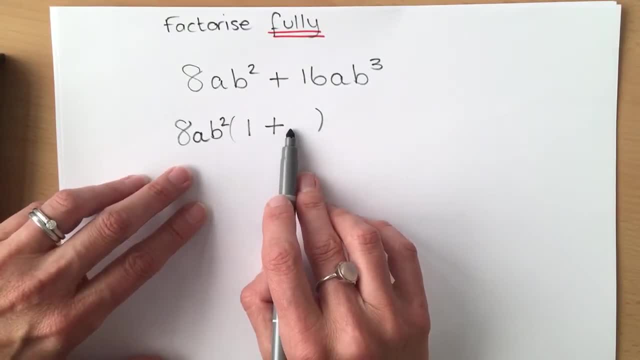 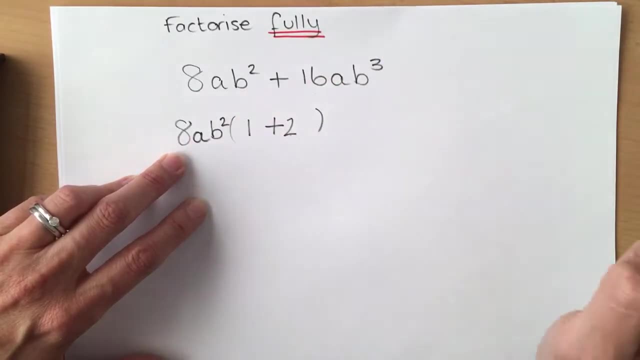 I need. let's start by the numbers. I need to multiply something by 8 to give me 16.. That something must be 2.. 2 multiplied by 8 is 16.. Then we're moving on to the a's. 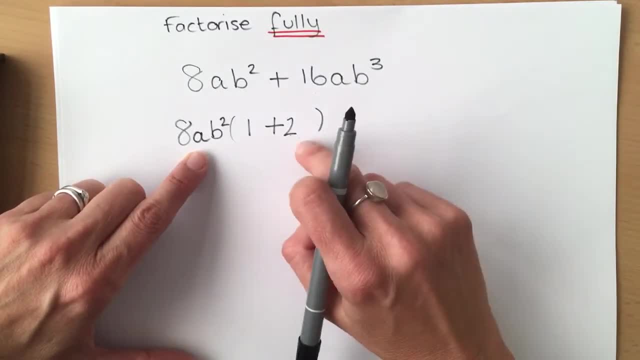 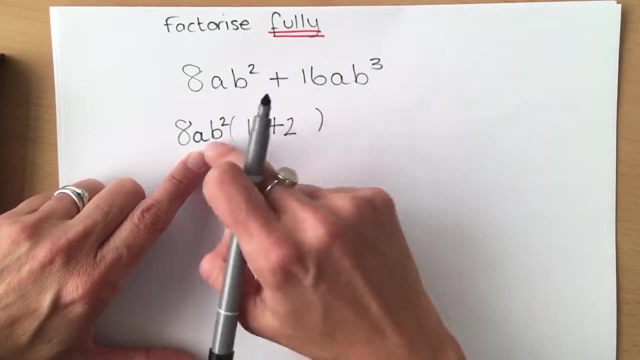 a times by something needs to give me a. Well, I don't need any more a, Because if I multiply it by another a a times a would be a squared. So I don't need to add another a. I already have enough a's here. 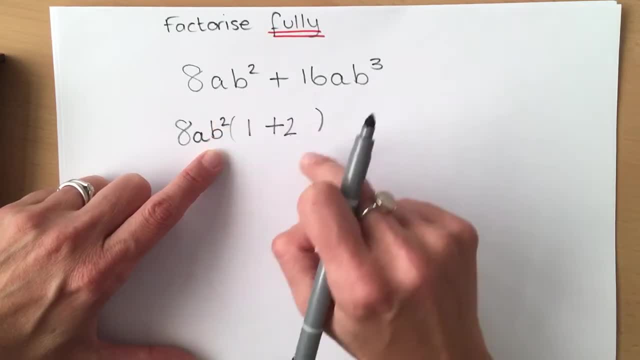 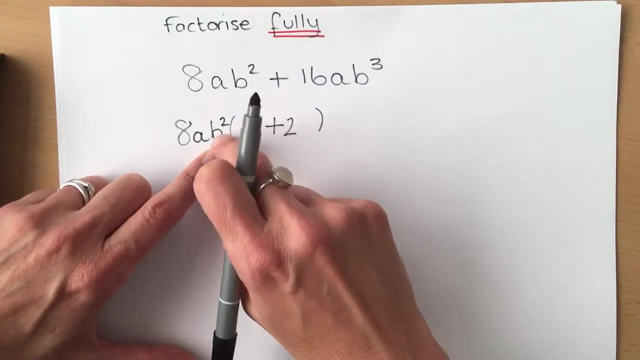 And then we move on to the b's, b squared times. something needs to give me b cubed. Now remember, when you multiply with powers, you add the powers I need to go from a b squared to a b cubed. So what I'm missing is b to the power 1.. 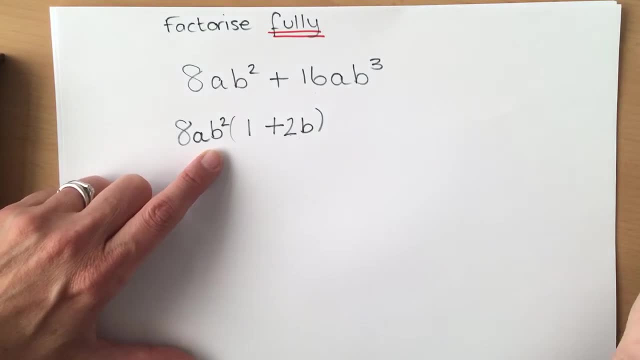 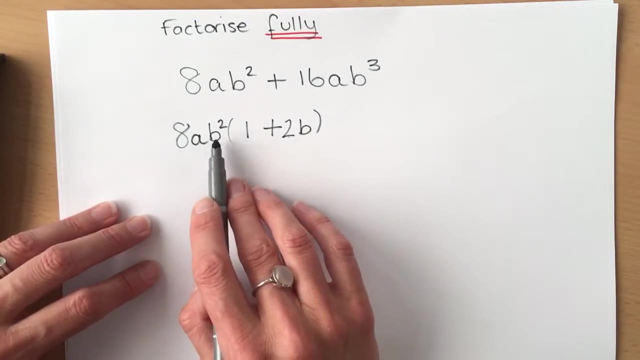 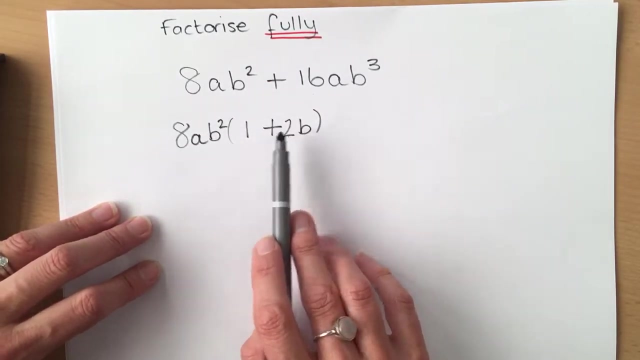 Or b. So let's see if this works by expansion: 8ab squared times 1 is 8ab squared, And then 8ab squared times 2b. The 2 and the 8 will give me 16a. 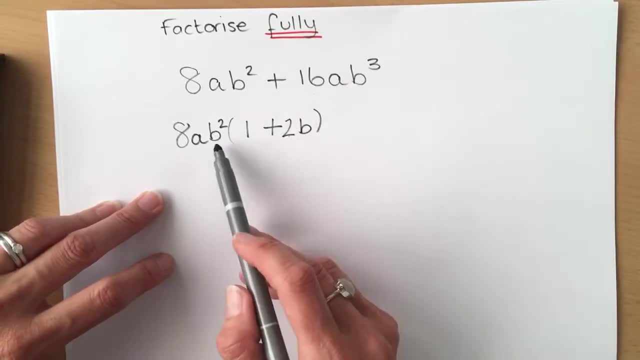 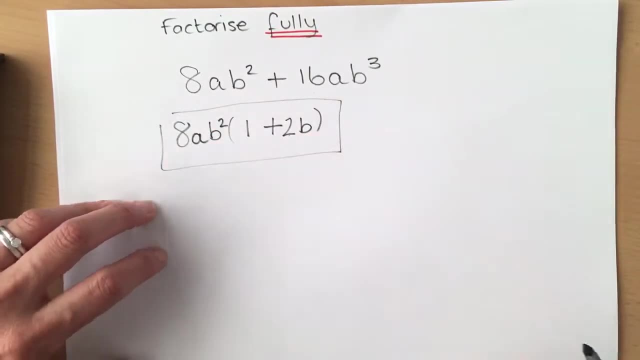 And no a there, but 1 is a And b squared times b is b cubed, So that works. That is my factorization of this expression, Thank you. 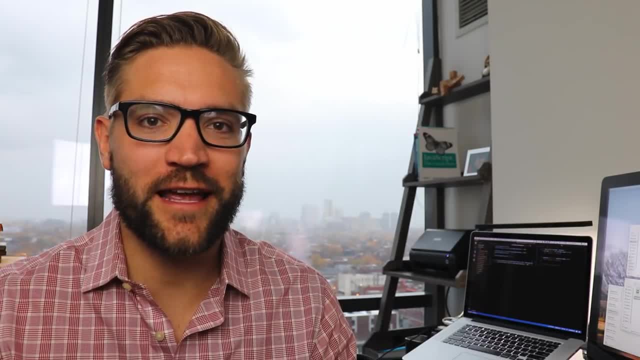 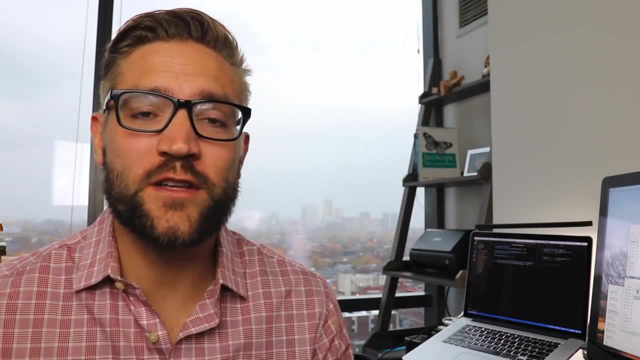 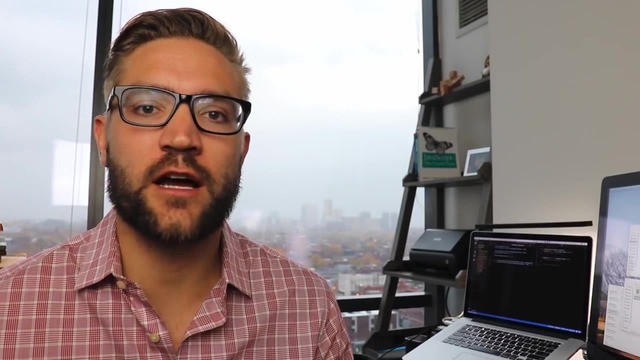 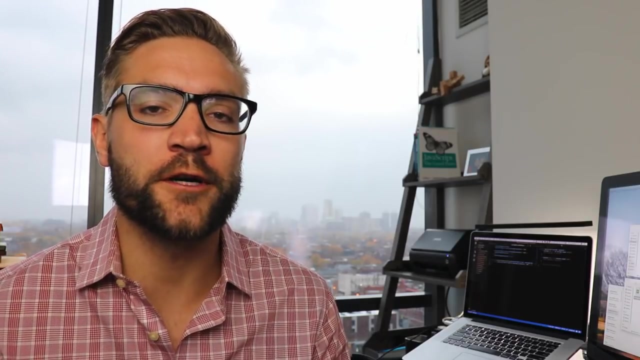 Hey everybody, what's going on? I'm Andy. I'm a self-taught software developer and in today's video we're going to be talking about unit testing, something I really love. It's near and dear to my heart, but this is going to be really important for anybody who is just getting started in software development, whether you've just discovered it, you're self-teaching or you're going to school. and even if you've just gotten your job and maybe you haven't been exposed to unit testing because your organization doesn't do that, It's really important to learn from the beginning because you never know, at one point in your career Maybe you'll be in a job interview where they will ask you about unit testing, and it's really good. 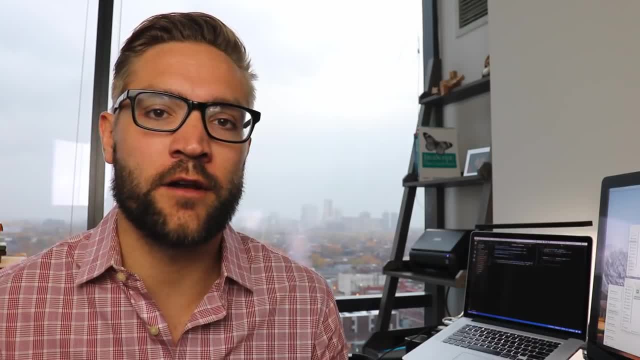 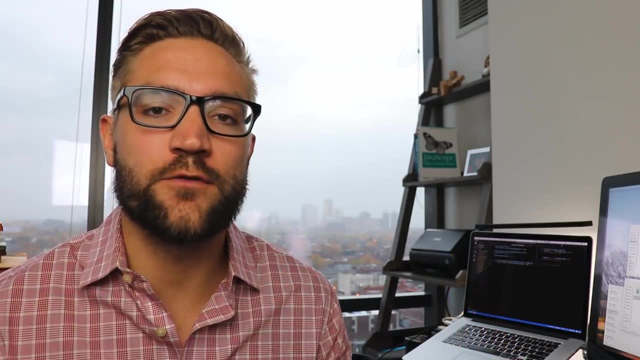 practice, to at least have the conceptual ideas down and be able to explain it to someone else. So I'm going to cover the basics. Unit testing to me is a wide or a deep subject that you can get into, so I'm only going to cover the basics. I'm definitely going to cover it more in the future.